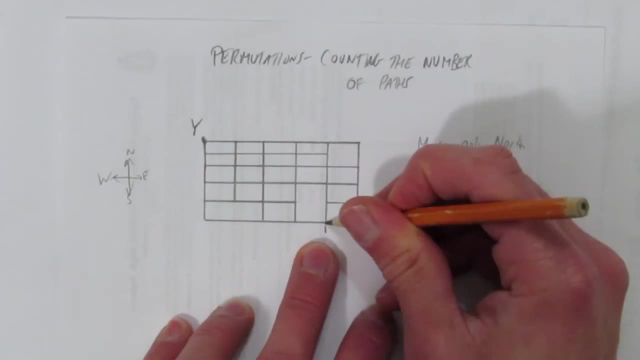 Okay, You go like this. There's no other way to arrive at this intersection. Same thing with this intersection. There's only one way to get there. You start here, go there, that's it. But this spot here you can either come up and go over or go left and go up. 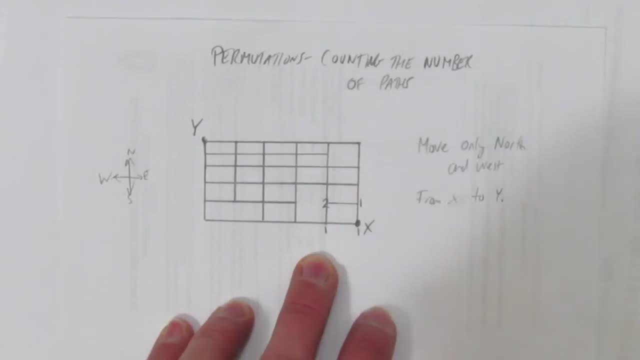 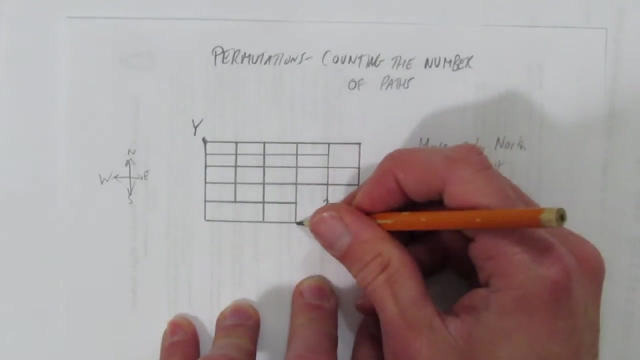 Either way is valid, so there's two ways to get there, And now we just keep doing the same sort of thing. It's based on the idea of Pascal's Triangle. How can you get to this intersection? The only way is to come west. There's one way. 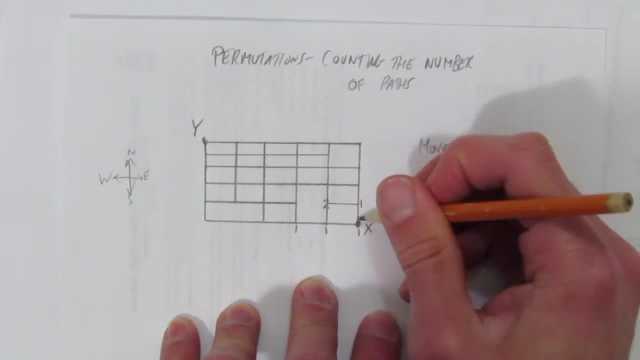 How do you get to this intersection? The only way is to go north. There's one way, But how do you get to this intersection? You can come from this one path or from these two paths. So you just add these two numbers together: Three. 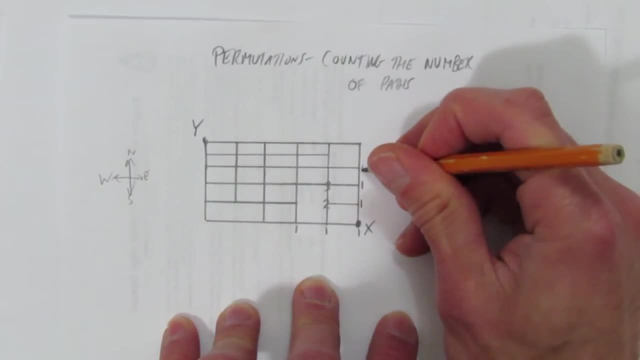 And as you practice it gets really easy. There's only one way to get here, but there are four ways to get here, Because you can either go this one path or this path, or this path or this path, And so don't bother counting all the paths, Just add the numbers. 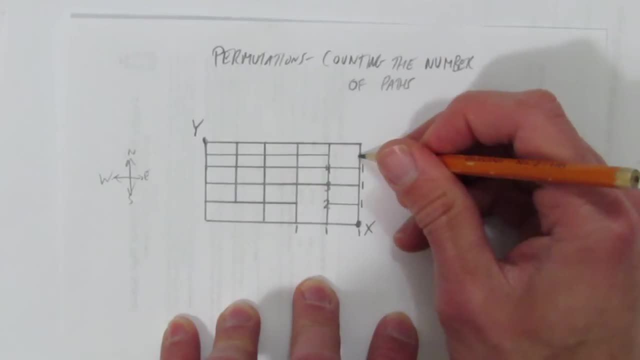 It gets tricky when you can't cross. for some people, For example, how many ways are there to get to this intersection? Well, the only way to get there is to come from below and go up. That is, you can only move north or west. You can't come west, so you've got to come north. 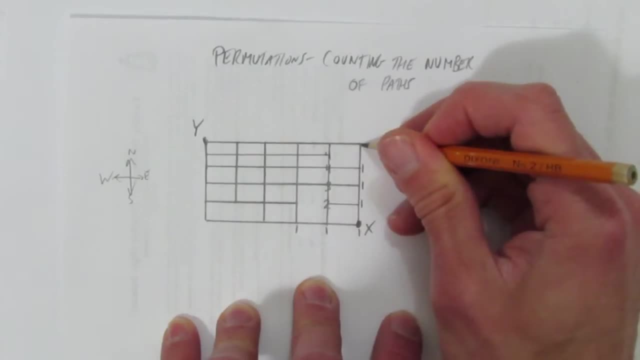 So this is a four. Up here. the only way to get here was to walk straight north every time, so that's a one. But to get to this spot you could either come from the one or come from the four. That's a five. 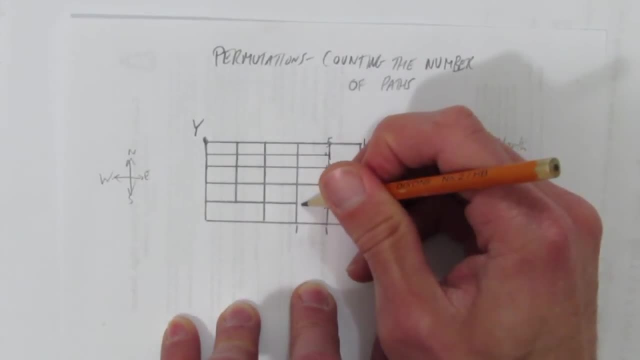 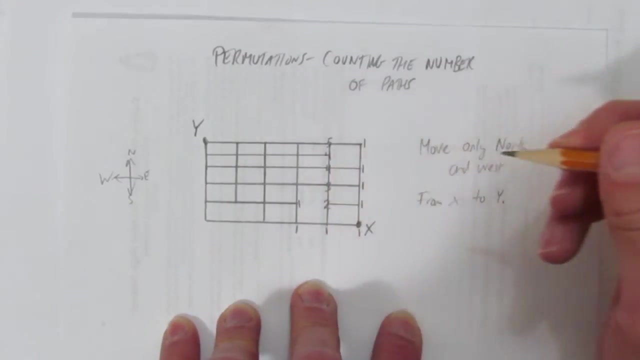 A lot of people make the mistake of using this two to get to this spot here. You can't. The only way to get there is to walk west, west and then north. There's only one way to get there, But to this spot there are four ways, Three plus one. 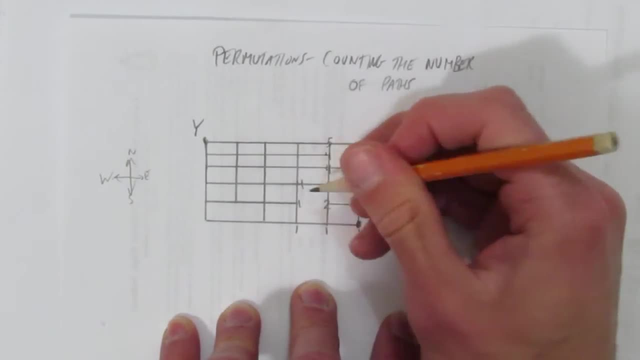 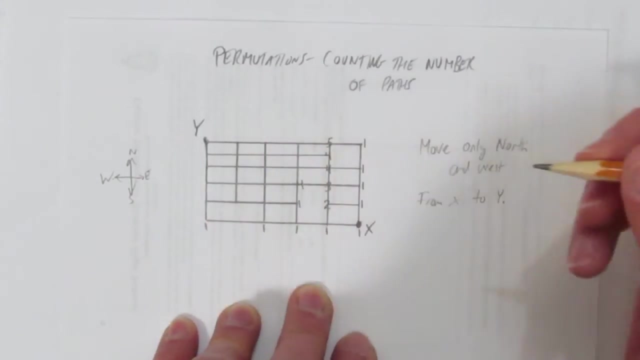 And you can do it in a column like that. It doesn't matter what order you go. Maybe you'd like to fill in this side here and say: Well, I only have one way to get here, and I only have one way to get here. 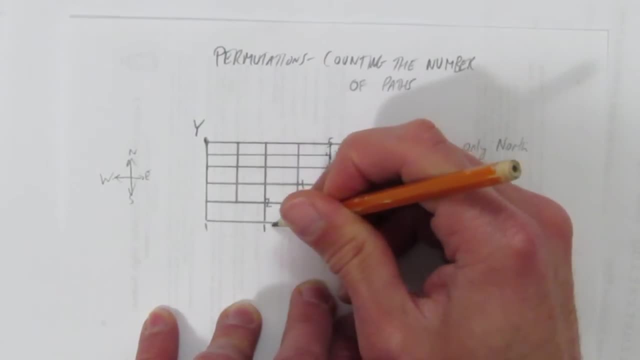 But this intersection, I have two ways. You can go this way, You can go this way- one, or this way, one. This intersection was a four, This was a two, So here's a six. Again, the order's up to you, but don't do an intersection until you have the two corresponding ones before it. 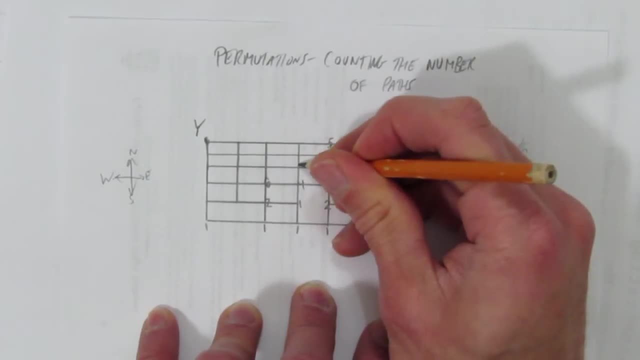 Four to get to this intersection. Four to get to this intersection. So that would mean this is an eight, This was a four, This is a twelve. Sorry, this is a four, This is an eight. So the answer: there are twelve ways to get to this intersection. 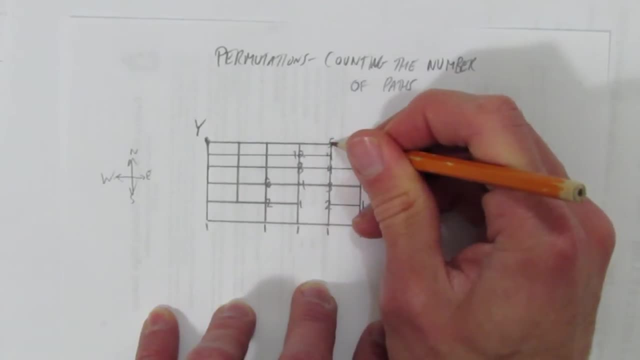 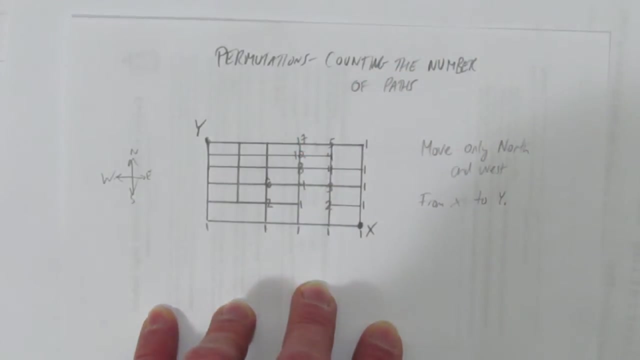 And this intersection, Twelve ways to get below it, Five ways to the right of it, So a total of seventeen ways to get to this intersection And, as you see, once you get it it gets fast. Add these two together to get this intersection Fourteen. 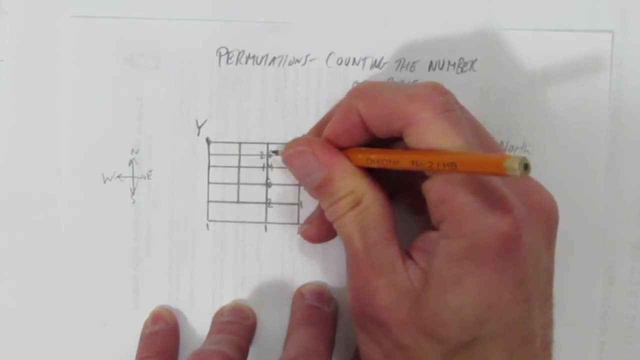 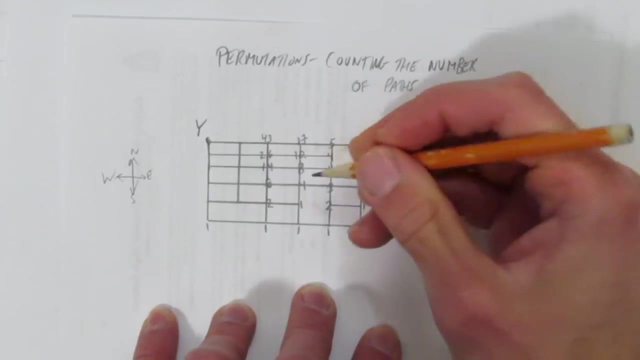 Add these two together to get this intersection Twenty-six. Add these two together to get this intersection Forty-three. So far, so good. I'm trying to get to Y. I'm just counting the paths. Here's another tricky one. 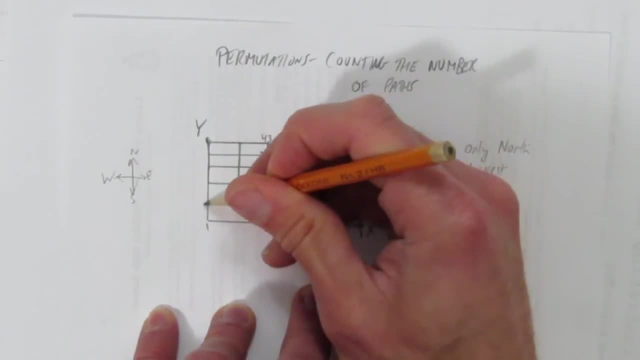 The only way to get to this intersection was to go west west, west west north. Oh no, Could have gone to here, you realize. So careful Almost made a mistake there. This isn't a one, because it could have come from here. 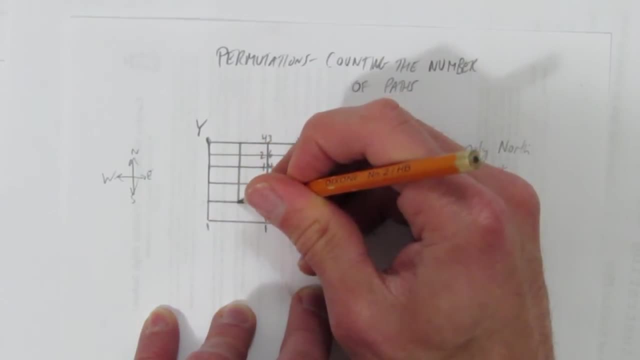 So let's figure out what this spot is. Well, the only way to get to this spot was to come from here. because you can't come from below, Had to come from the two, So there's only two ways to get here. 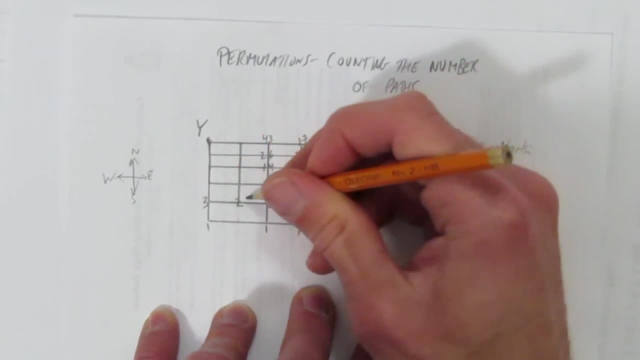 But there's three ways to get here. Two and six to get here Makes eight ways to get here. Fourteen and eight makes twenty-two ways to get here. Twenty-two and twenty-six means there's twenty-eight ways to get here And twenty-eight. 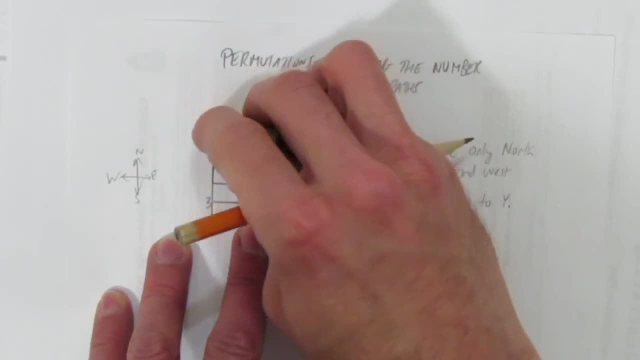 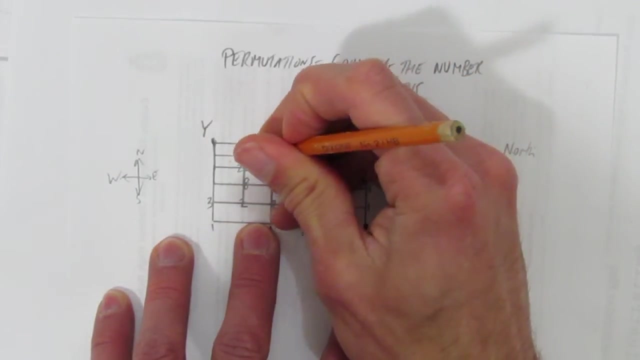 Oh, that doesn't make sense. Twenty-eight, Twenty-six plus twenty-two is forty-eight. This is forty-eight ways to get here. Forty-eight plus forty-three is ninety-one, So ninety-one ways to get here. So I know ninety-one ways to get here.